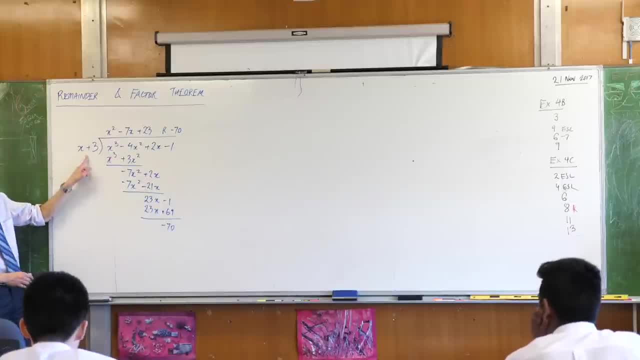 I want to remind you this is not new stuff. This thing that you're dividing by what's this called? Does anyone remember? It's the divisor. Since it's the divisor, let's call it d of x, This here, this polynomial, the one being divided by what's it called? It's. 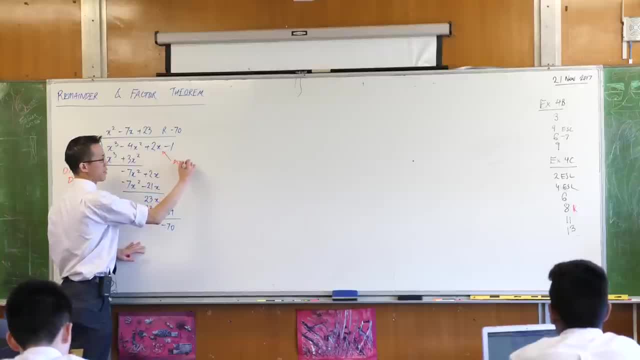 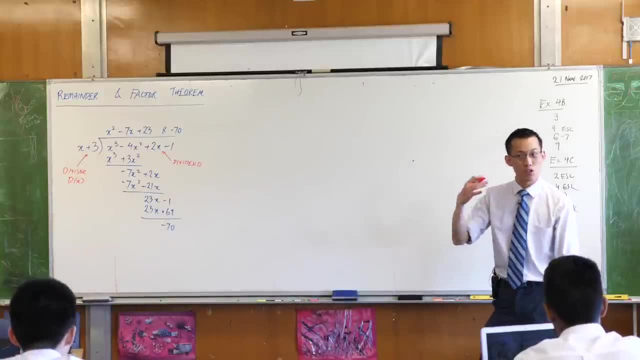 called the dividend. very good, Quite an uncommon word. we hardly use it. I mean, we don't use it. It's sort of been taken over by its financial meaning. nowadays, The dividend is the polynomial you started with. so the polynomial you start with is usually called. 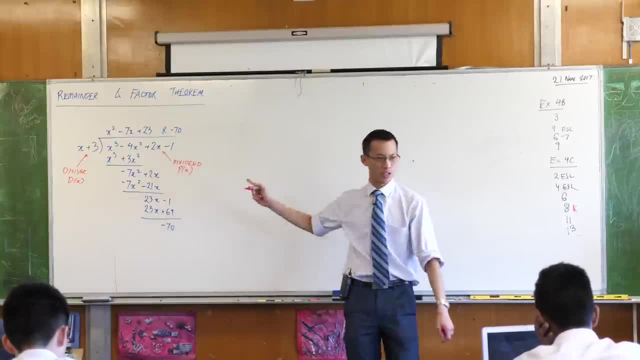 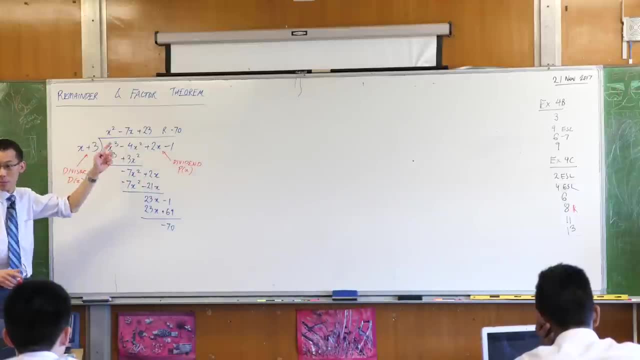 p. I might as well call it that, because I can't call it d anyway, because I've already used that letter. What you get left with at the top is your answer, which is comprised of two components. There's this part over here which is the starts with a, q. It's. 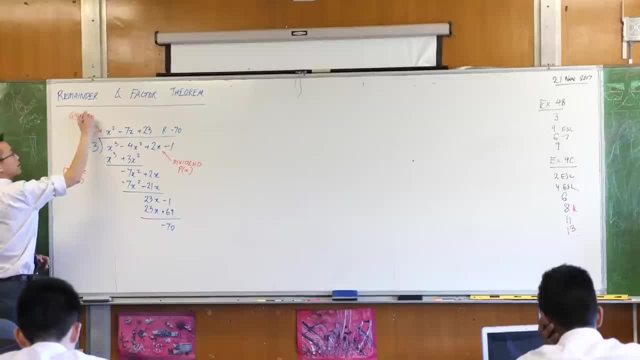 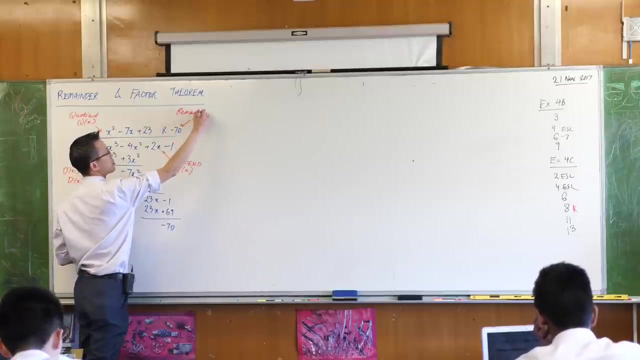 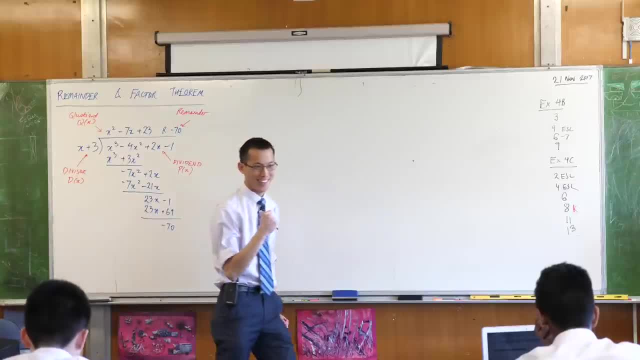 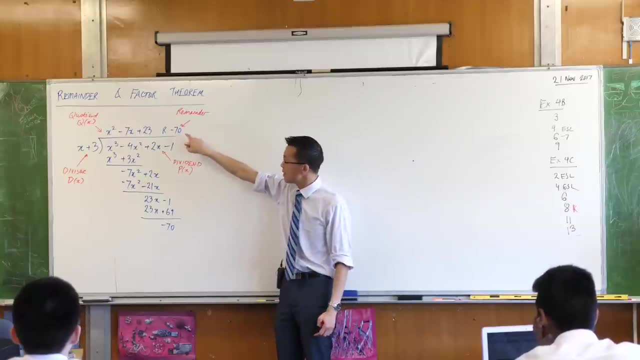 there's this number here, But for those of you who were faithful and were here on Wednesday morning, you might remember this. remainder isn't always just a number. It's not always just a number. In this case, it's a number because I was dividing through by something linear. 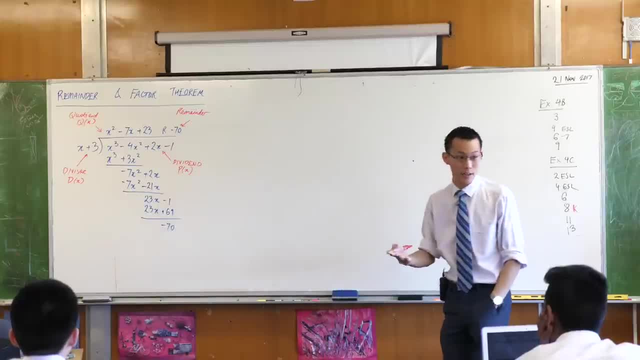 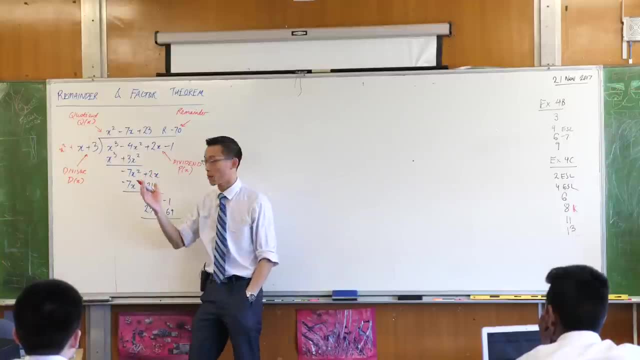 But if my divisor was not linear, if my divisor was, say, a quadratic- okay, if I divided this cubic by, you know, x squared plus x plus 3, I could have done that. that would have been fine. If you have a quadratic divisor, your remainder might not be just the number. 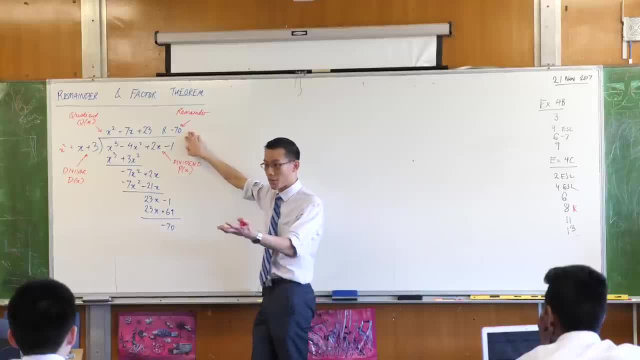 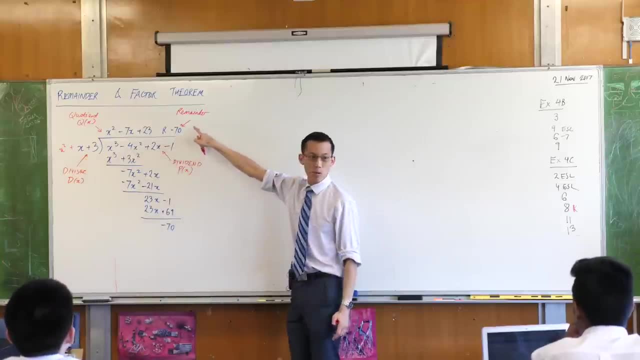 What might it be? It might have some x terms in there, right? What we saw was the degree here is going to be one more than the degree here. okay, Or another way of saying it is that the degree of your remainder is always one less than. 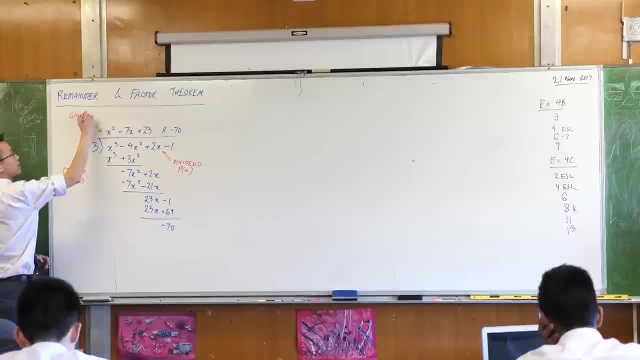 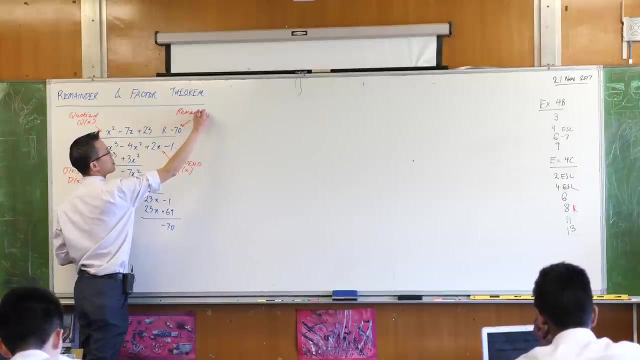 the quotient, The quotient, The quotient. So I guess we can call that q of x, And that leaves the final piece, the remainder. Now a quick note. I've said let's call each of these pieces d of x, p of x, q of x, and 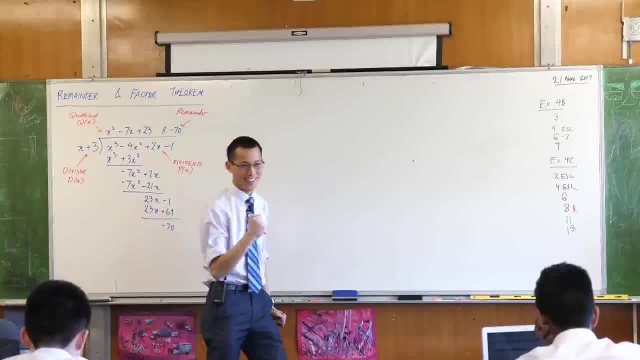 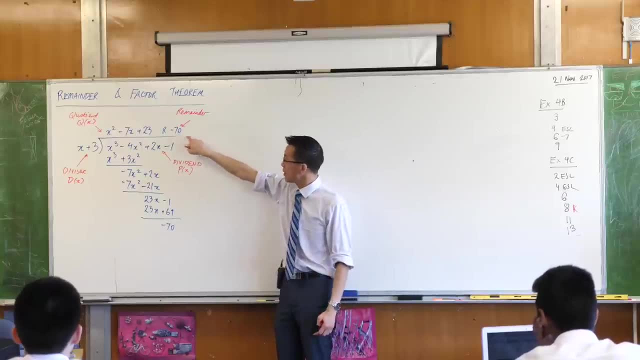 then there's this number here, But for those of you who were faithful and were here on Wednesday morning, you might remember this remainder isn't always just a number. it's not always just a number- In this case a number- because I was dividing through by something linear. 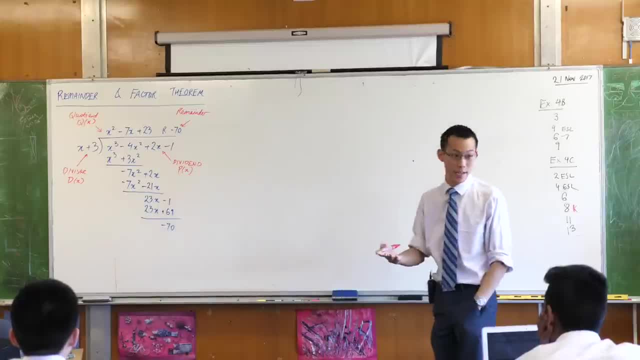 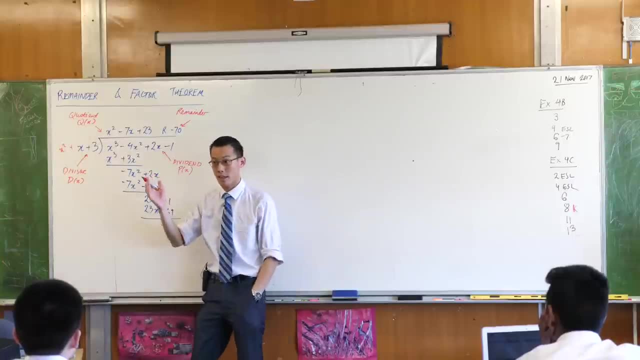 But if my divisor was not linear, if my divisor was, say, a quadratic, if I divided this cubic by x, squared, plus x plus 3, I could have done that. That would have been fine. If you have a quadratic divisor, your remainder might. 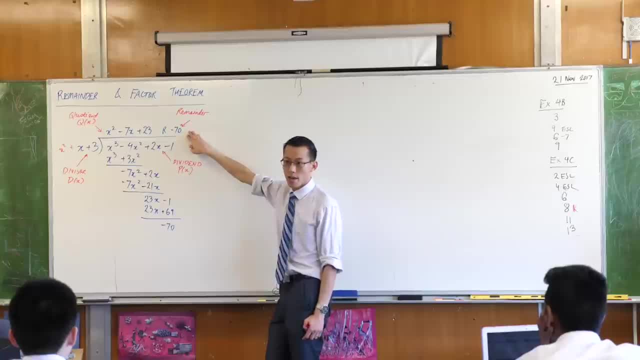 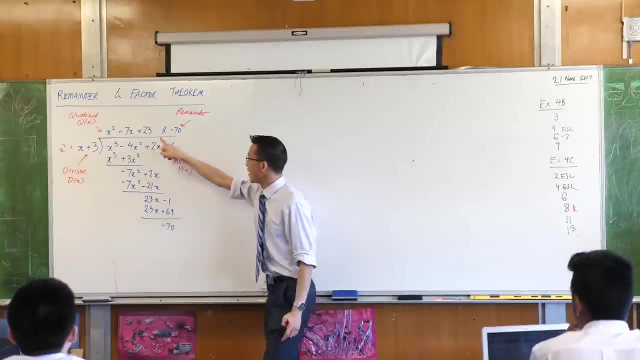 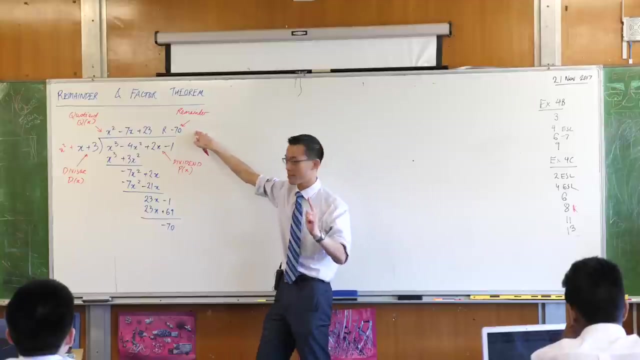 not be just the number? What might it be? It might have some x terms in there. What we saw was the degree here is going to be one more than the degree here, Or another way of saying it is that the degree of your remainder is always one less than the. 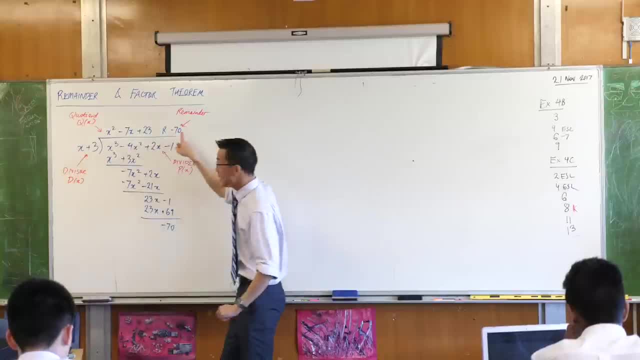 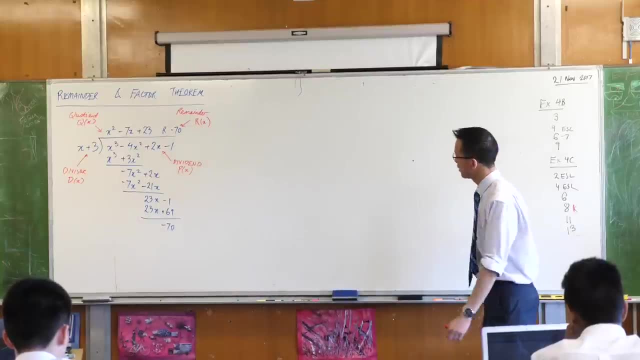 degree of your divisor. So therefore, this here, the remainder is itself also a polynomial. In this case it's just the constant polynomial. So d, p, q and r, these are the pieces in here. What I want us to do is just write it again. but in general, 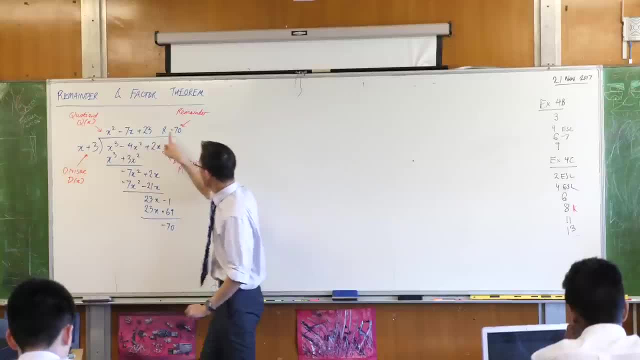 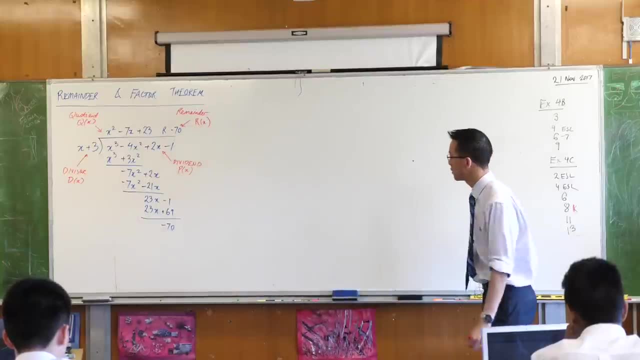 the degree of your divisor. okay, So therefore this here, the remainder, is itself also a polynomial right. In this case it's just the constant polynomial. okay, So d, p, q and r, these are the pieces in here, right? 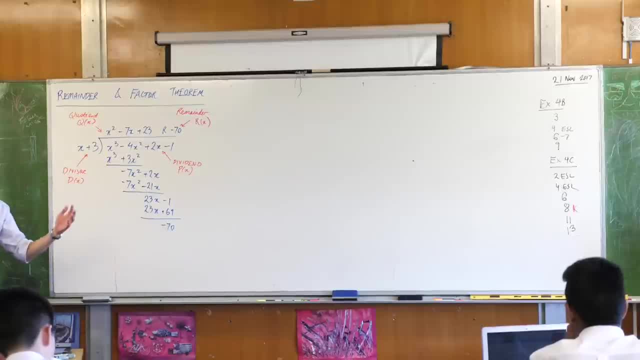 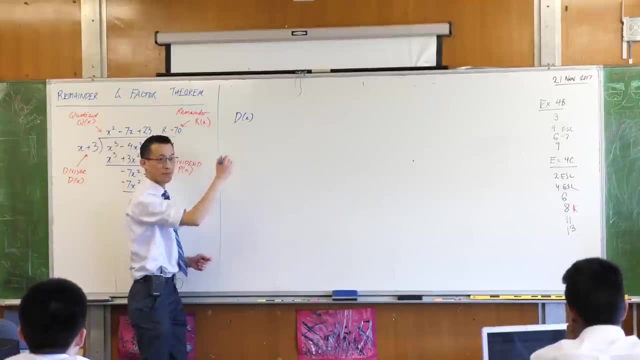 What I want us to do is just write it again, but in general terms, not for this specific example, right, But generally speaking. we always have the divisor over here, right? We have the original polynomial, the dividend underneath, and then what you get left with. 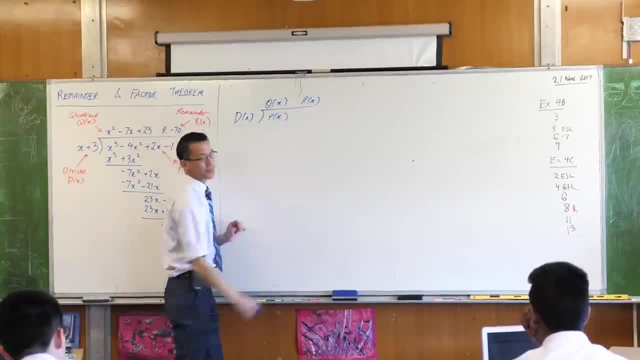 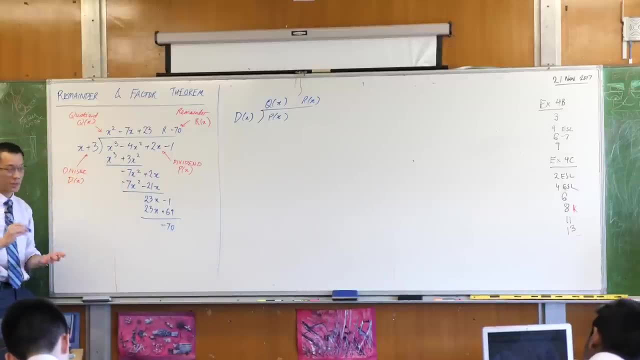 is your quotient and your remainder. okay. Now what I'd like us to do is look at this thing here and make a statement about all of this from this working, And we'll come up with an equivalent statement. We'll come up with an equivalent statement over here. 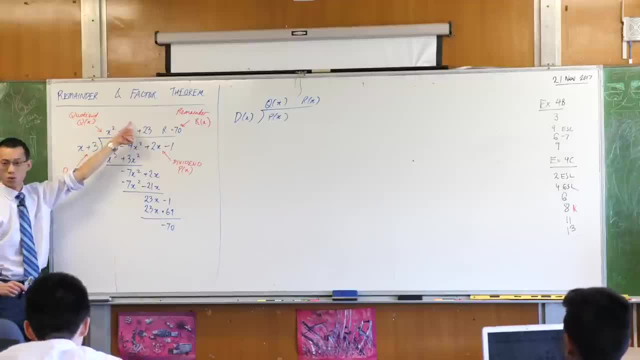 If I've divided this cubic by this linear thing and gotten this quadratic and this remainder, then I can say that the original polynomial p x, cubed minus 4x, squared plus 2x minus 1, it equals to. I can say it in terms of all these other pieces, right? 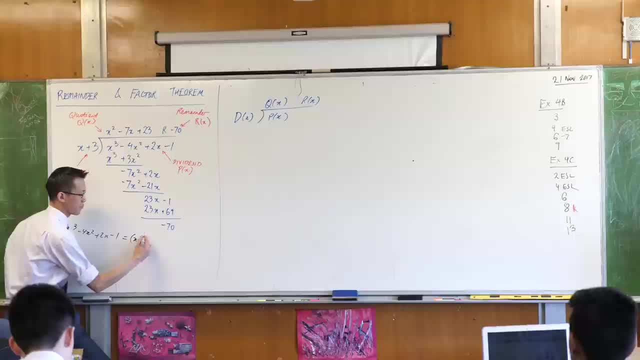 In fact, I'm even going to say it in order: It's the divisor multiplied by the quotient. And then how does the remainder come into play? Okay, It comes into play, plus the remainder, which in this case is minus 70, okay. 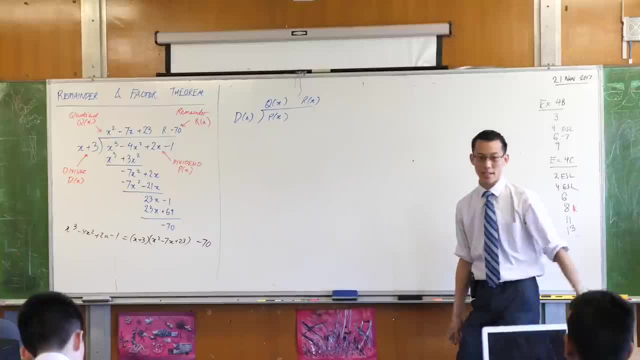 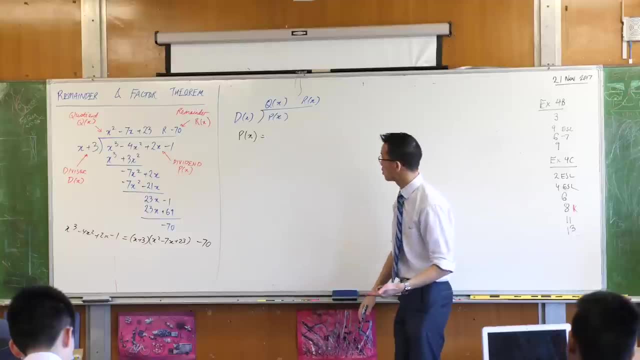 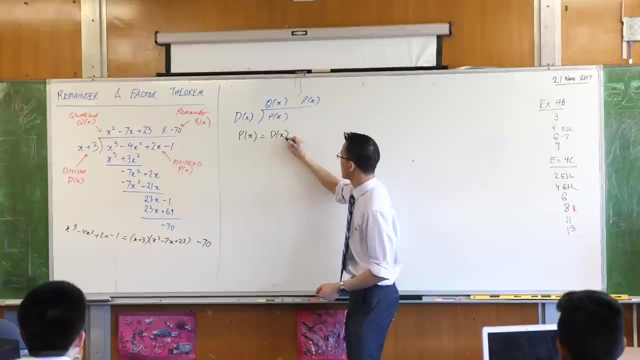 So I can state that, in general terms, for any polynomials being divided in the following way, The original polynomial p, what it equals to is- let's write this carefully- the divisor times the quotient plus the remainder. Is that okay? Divisor quotient, remainder, all happy. 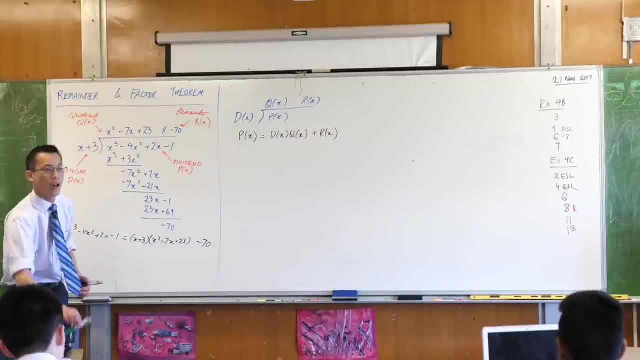 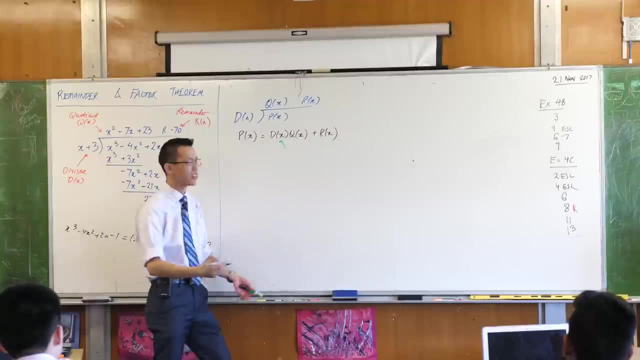 Let's make that statement again about the oops, wrong color, about the degrees, because that's going to become quite important in a second. If this divisor here has a degree of, I mean, it can have any degree, can't it right? 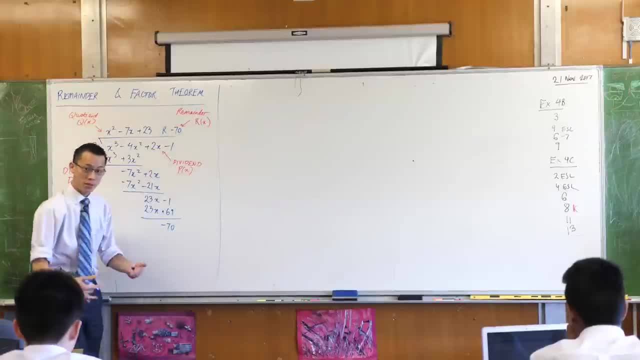 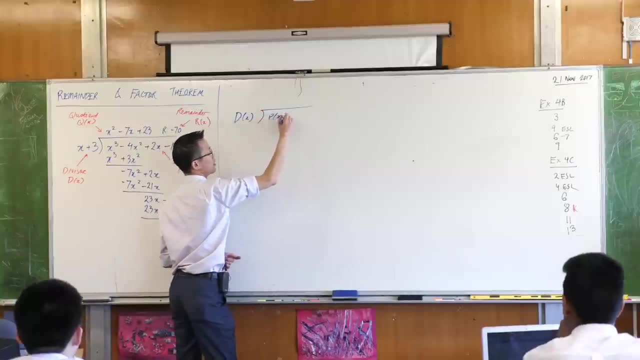 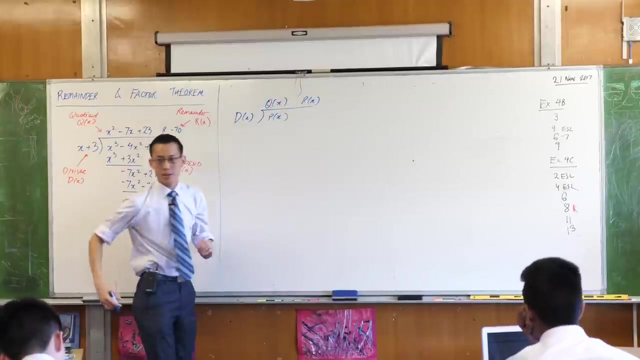 terms, not for this specific example, But generally speaking. we always have the divisor over here, we have the original polynomial, the dividend, underneath, and then what you get left with is your quotient and your remainder. Now, what I'd like us to do is look at this thing here and 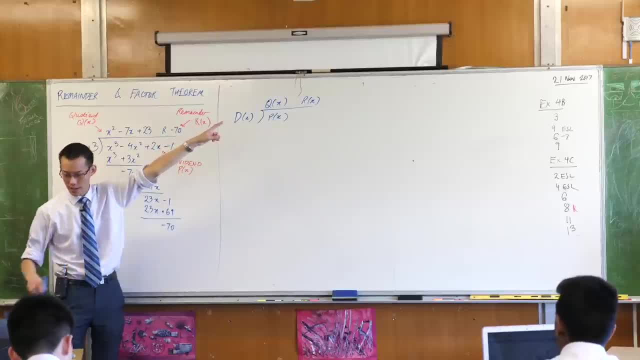 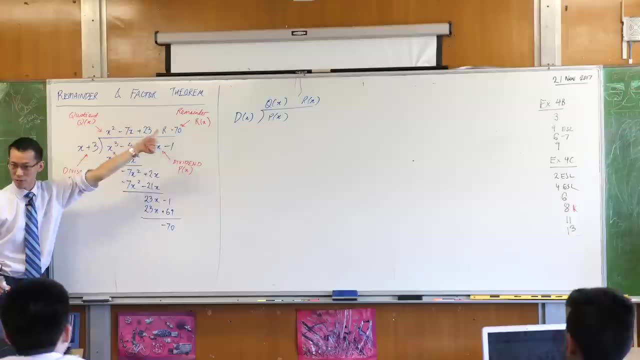 make a statement about all of this from this working and we'll come up with an equivalent statement over here. If I've divided this cubic by this linear thing and gotten this quadratic and this remainder, then I can say that the original polynomial p x cubed minus 4x, squared plus 2x. 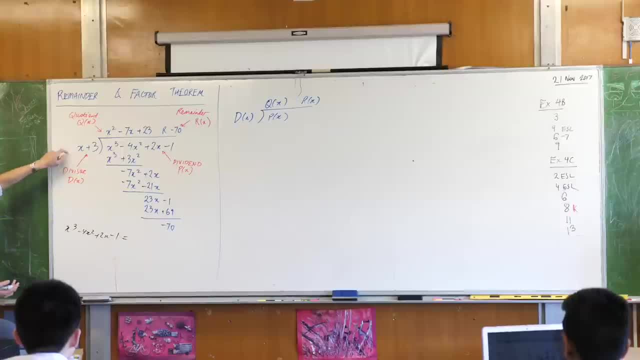 minus 1, it equals to- I can say it in terms of all these other pieces, In fact, I'm even going to say it in order: It's the divisor multiplied by the quotient, And then how does the remainder come into play? 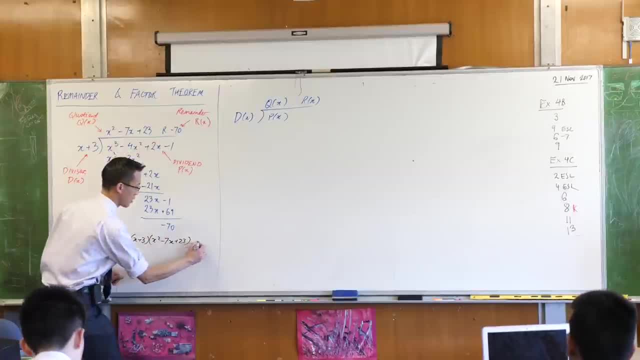 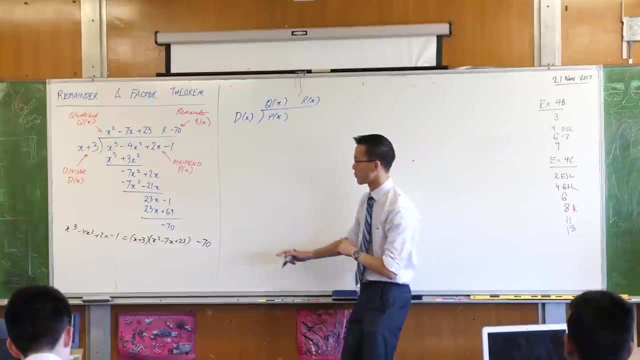 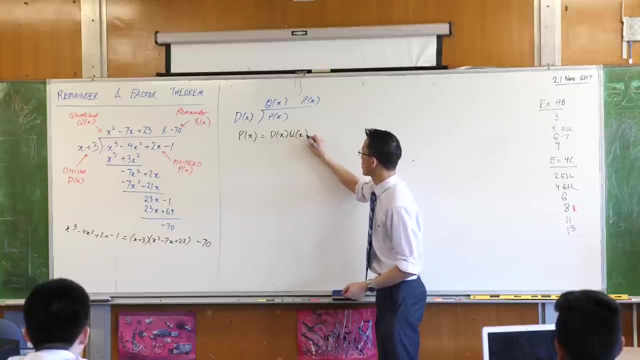 Plus the remainder, which in this case is minus 70.. So I can state that, in general terms, for any polynomials being divided in the following way, The original polynomial p, what it equals to is- let's write this carefully- the divisor times the quotient plus the. 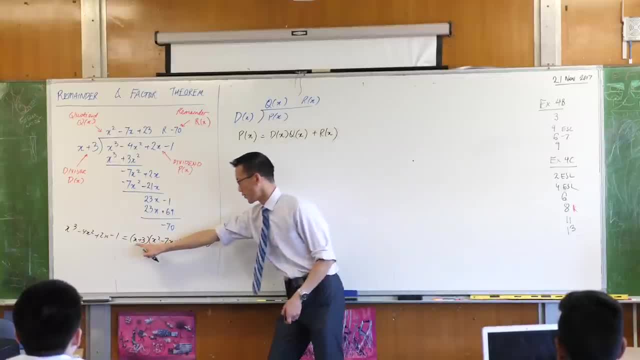 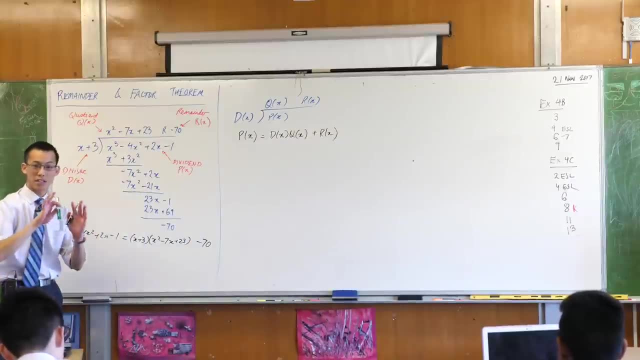 remainder Is that OK. Divisor quotient remainder: All happy. Let's make that statement again About the degrees, because that's going to become quite important in a second. If this divisor here has a degree of, I mean, it can have. 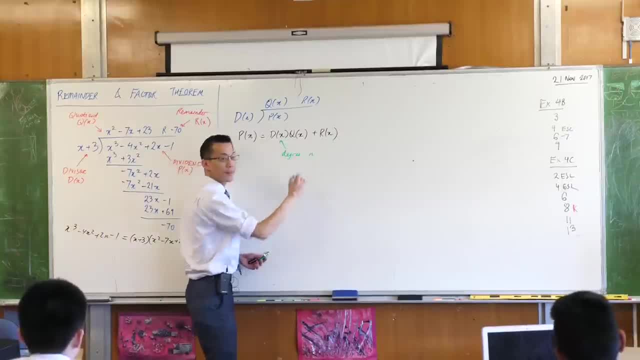 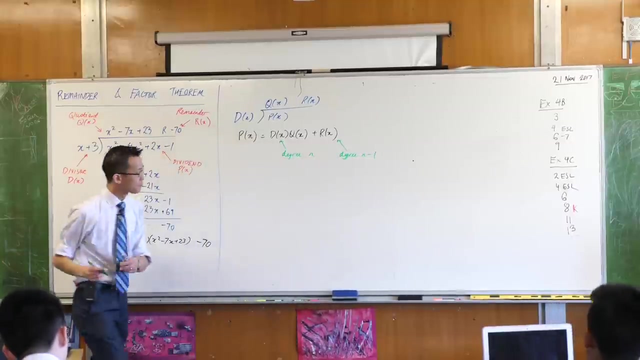 any degree, can't it? Let's say degree n. What that will mean is: the remainder over here has a degree of what? Yeah, one less will be n minus 1.. OK, So I want to look at the specific example and you'll see why we're doing this later. 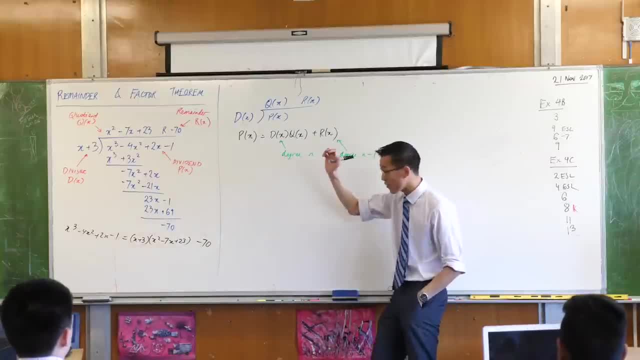 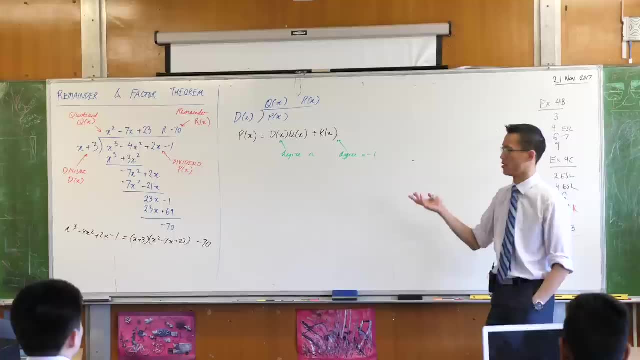 When we have a linear divisor, we have this a whole lot. It's very, very common. It's the most common thing we have to do. We only show you how to do quadratics and cubic divisors, just because we can, but it's not that useful. 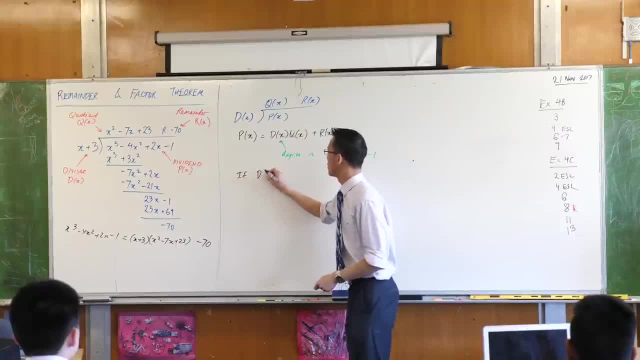 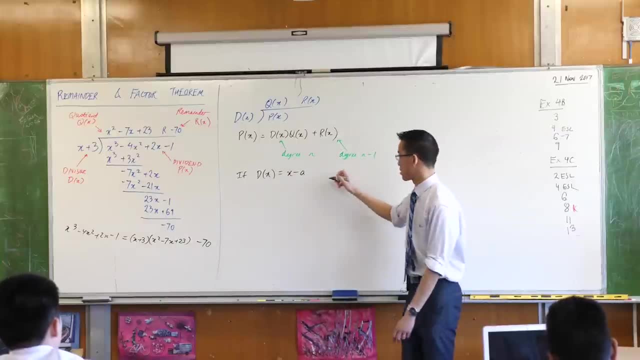 If I have a divisor that is monic and linear- these are the most common ones we deal with- where a is a constant. So if I have a divisor that is monic and linear, then I can rewrite this statement with some interesting sort of. 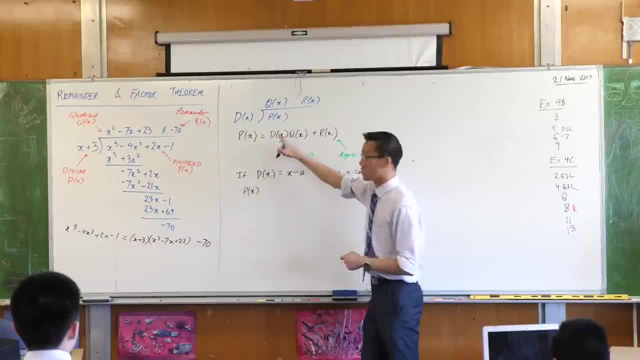 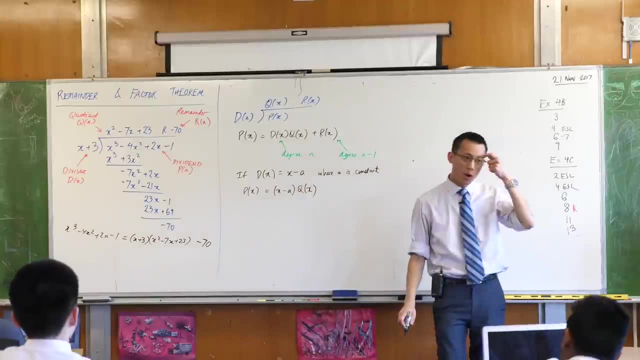 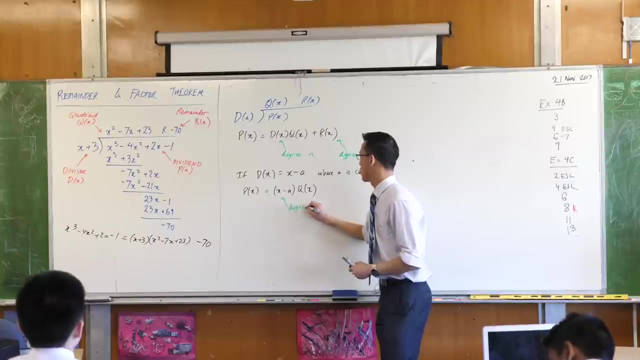 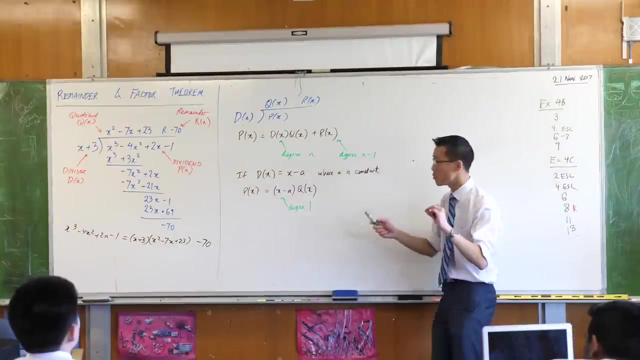 consequences. I can say that p of x is the divisor which is x minus a times the quotient. And because I have a divisor that is degree 1,, what will be the degree of my remainder? It will be 1 minus 1,, which is 0, which is exactly what we. 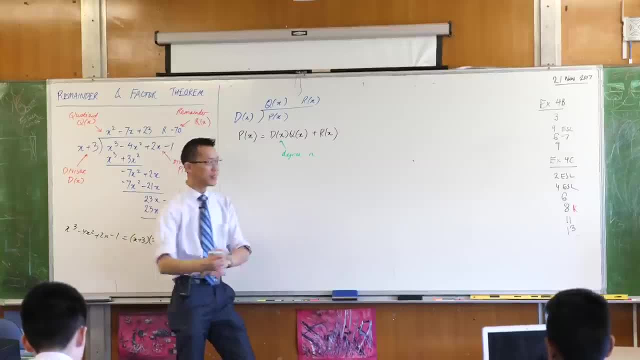 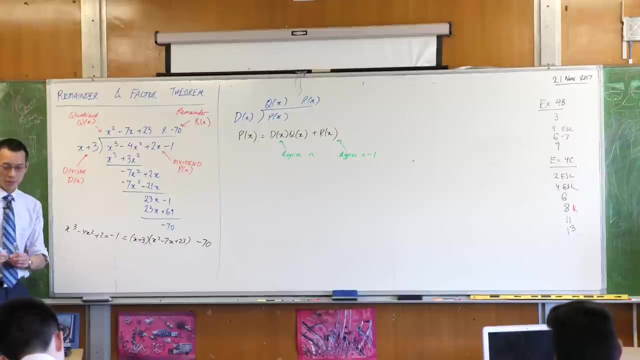 Let's say degree n. What that will mean is the remainder over here has a degree of what. Yeah, one less will be n minus 1. Okay, Okay. So I want to look at the specific example and you'll see why we're doing this later. 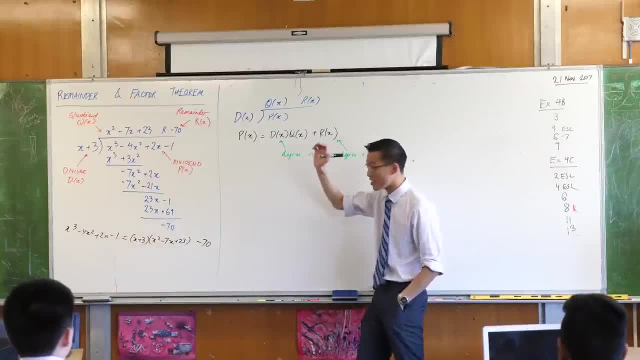 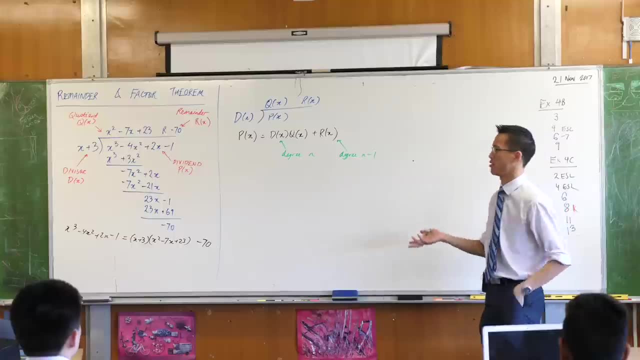 When we have a linear divisor, we have this a whole lot. It's very, very common. It's the most common thing we have to do. We only show you how to do quadratics and cubic divisors, just because we can, but it's. 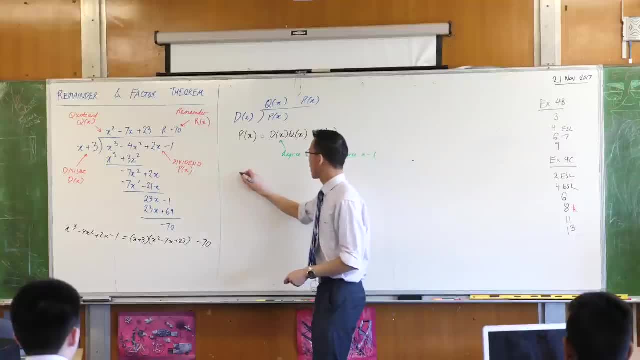 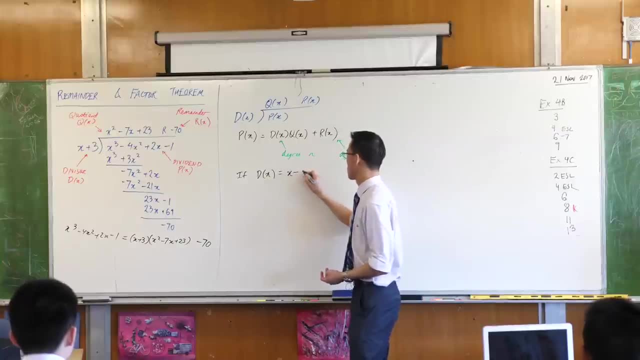 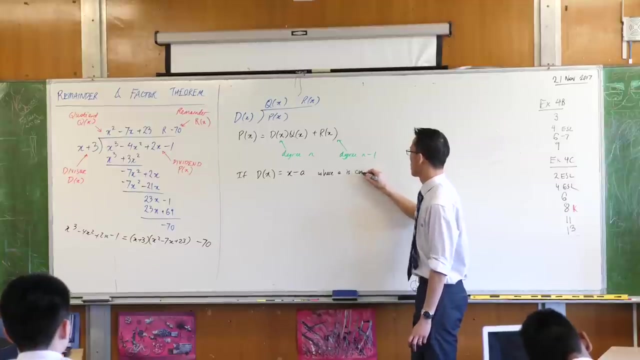 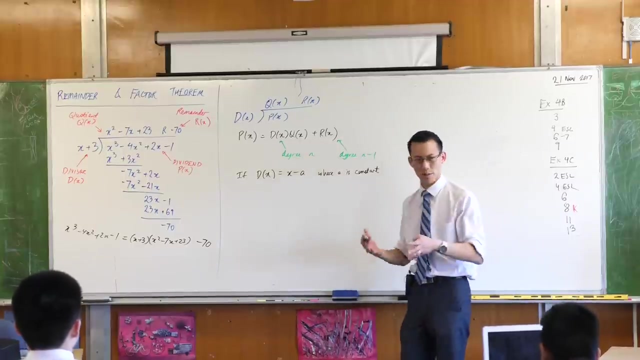 not that useful. okay, If I have a divisor that is monic, Monic and linear- These are the most common ones we deal with. okay, where a is a constant, then I can rewrite this statement with some interesting sort of consequences, right? 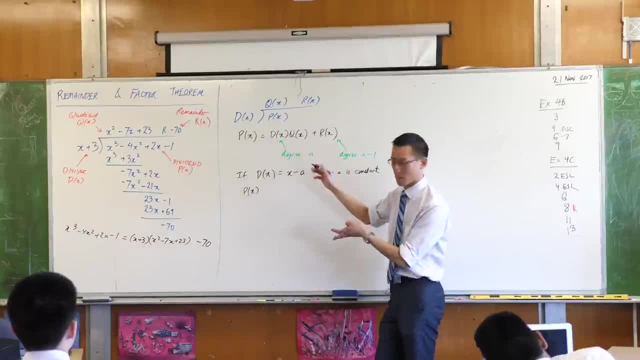 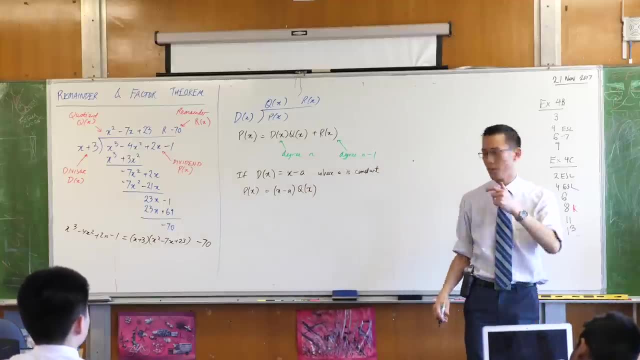 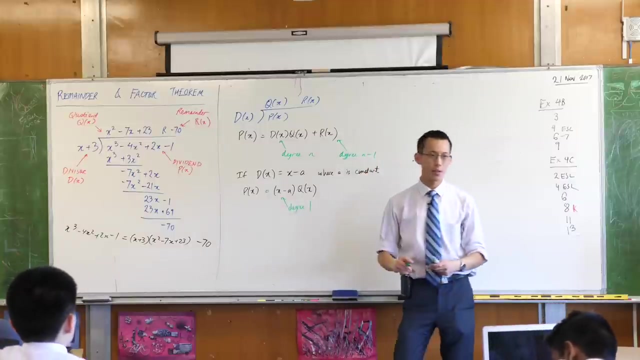 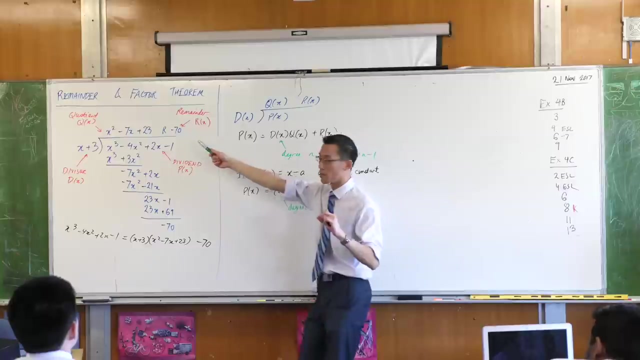 I can say that p of x is the divisor, which is x minus a times the quotient, and because I have a divisor, Hmm, That is degree 1.. What will be the degree of my remainder? It'll be 1 minus 1, which is 0, which is exactly what we sort of are used to getting. 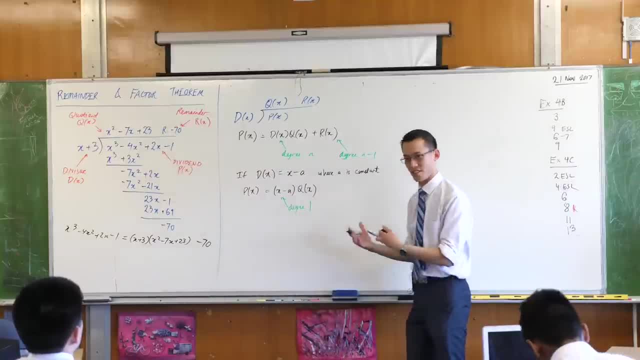 You see that That's a polynomial of degree 0, okay, So, since it's just a number, it's degree 0, I'm going to say plus r and I don't need to say any x's here. It's actually independent of x. 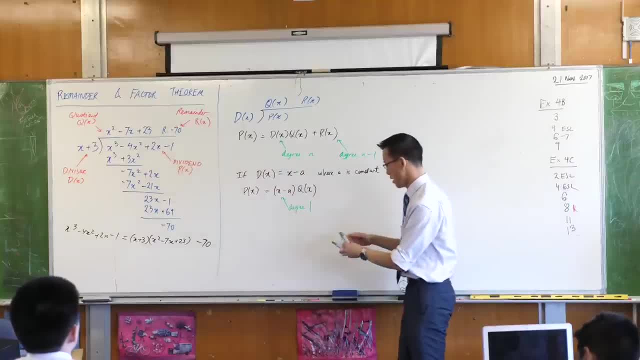 sort of are used to getting. You see that That's a polynomial of degree 0. So since it's just a number, it's degree 0, I'm going to say plus r And I don't need to say any x's here. 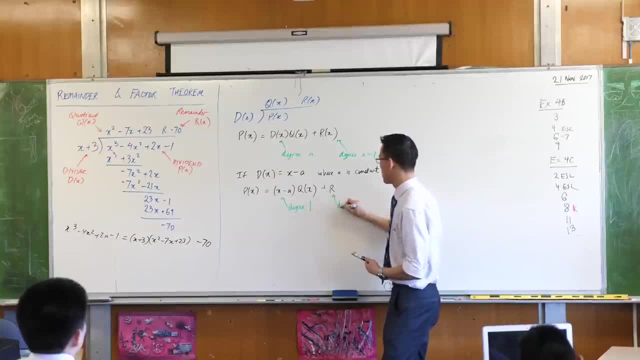 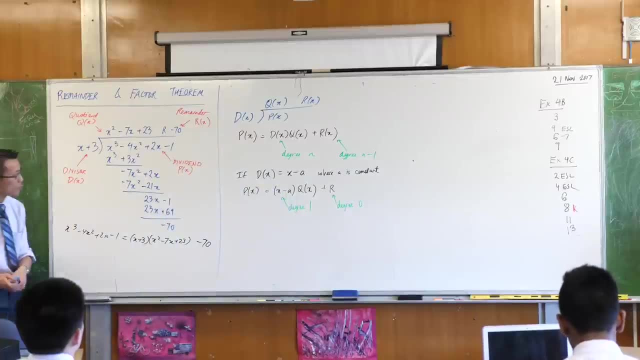 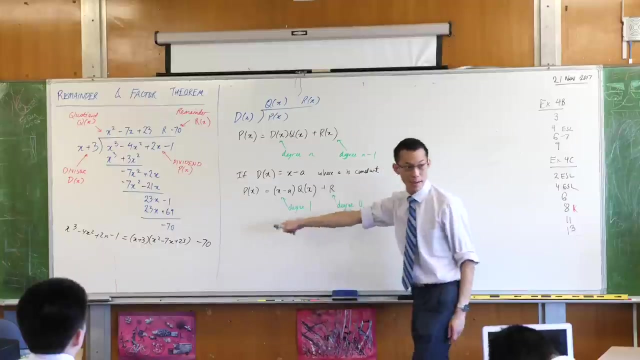 It's actually independent of x, It's just a constant. So this guy here is degree 0.. Now watch what happens. I can really quickly find out what the remainder of something is, Rather than by going through this whole long process. you can see the remainder is the last. 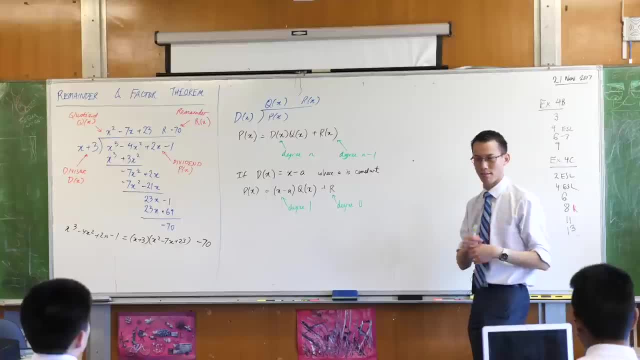 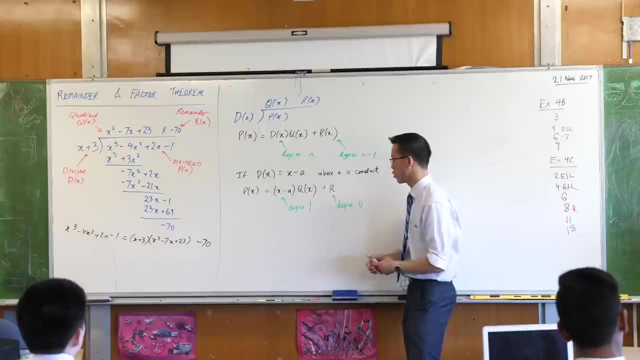 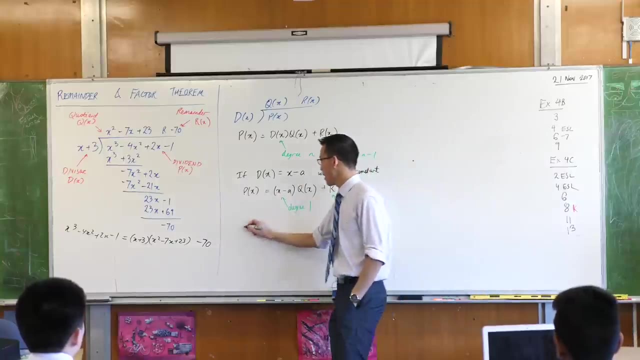 thing you find out If I want to. if it's useful to me- spoilers, it will be. if it's useful to me, I can find out the remainder immediately, without going through this whole process by making x equal to a Watch. 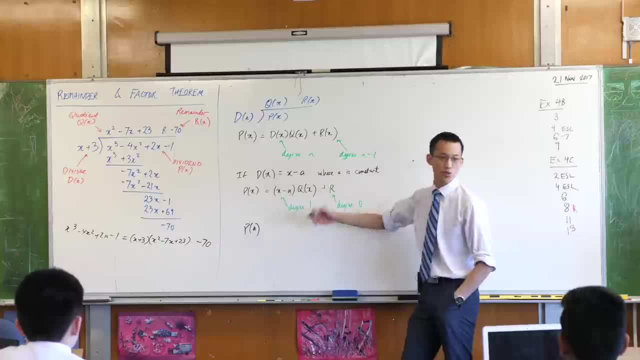 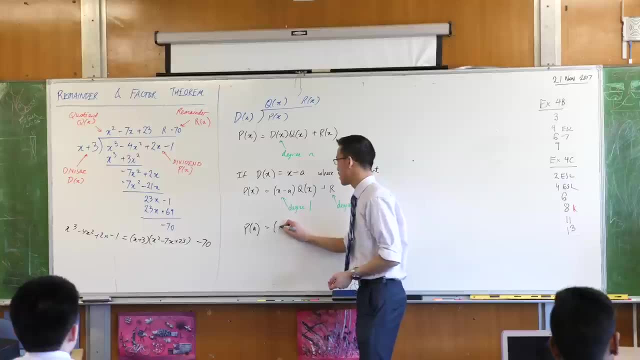 If I substitute in x equals a. this is just using function notation. then what happens? Well, I'm going to put in an a everywhere. I see an x. I see it two places. I see it there once and I see it there twice. 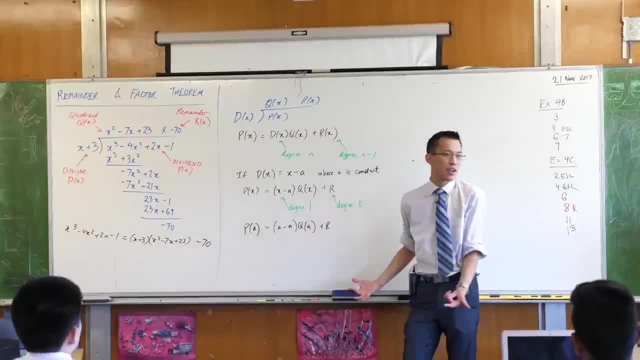 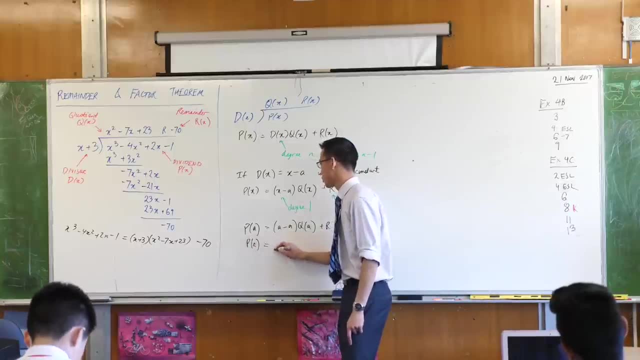 That, OK. And then, of course, the remainder is independent of x, So it just sits out there on the side. Well, this is just 0. So what I find is that p of a equals the remainder. So what this means is, if I come back over here, this: 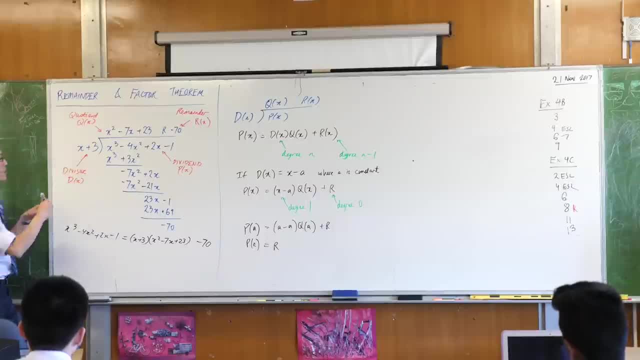 original example that we did. if this thing is my x minus a, what is a in this case? Look carefully. Yeah, it's negative 3, isn't it? Because it's x minus negative 3 will give me this divisor. 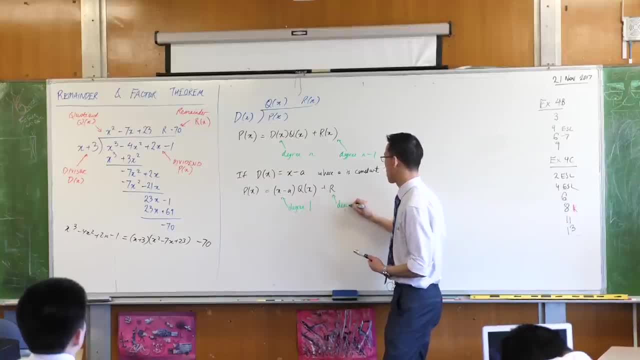 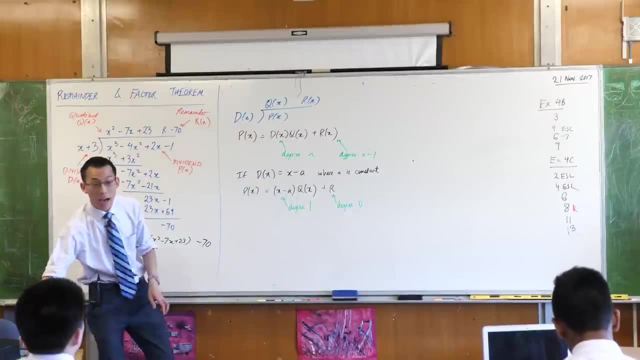 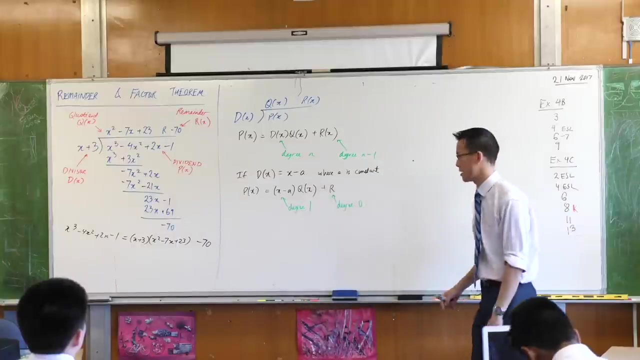 It's just a constant. So this guy here is degree 0.. Okay, Now watch what happens. I can really quickly find out what the remainder of something is, rather than by going through this whole long process. You can see, the remainder is the last thing you find out. 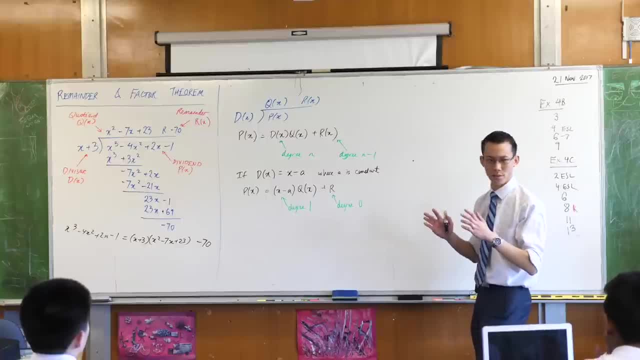 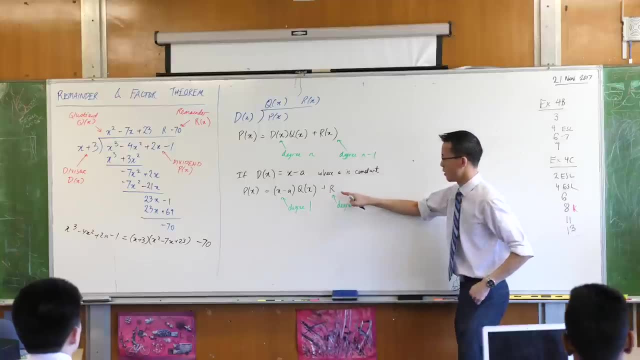 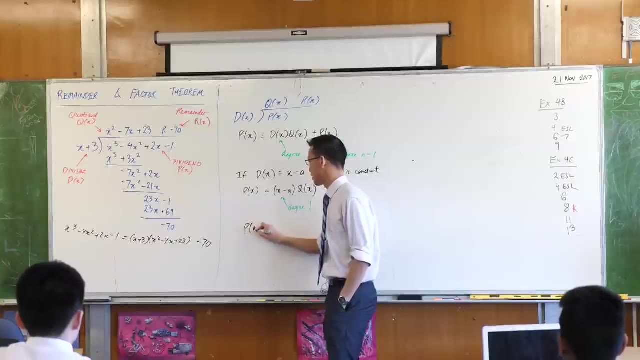 If I want to, if it's useful to me, spoilers it will be. if it's useful to me, I can find out the remainder immediately, without going through this whole process, by making x equal to a Watch, Watch, Watch. 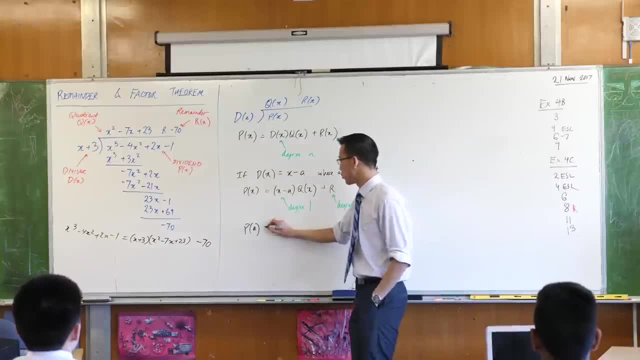 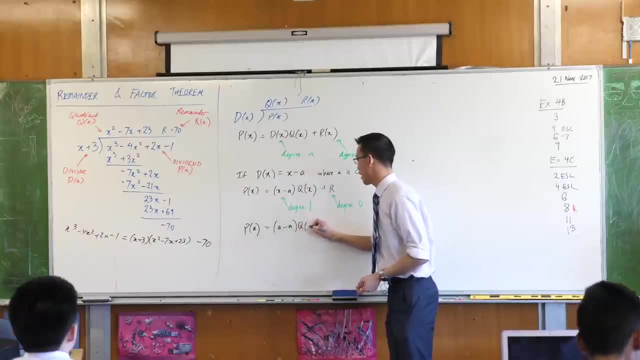 So this is an x-squared x equals a Right. This is just using function notation, right, Then what happens? Well, I'm going to put in an a everywhere. I see an x. I see it two places. I see it there once and I see it there twice. 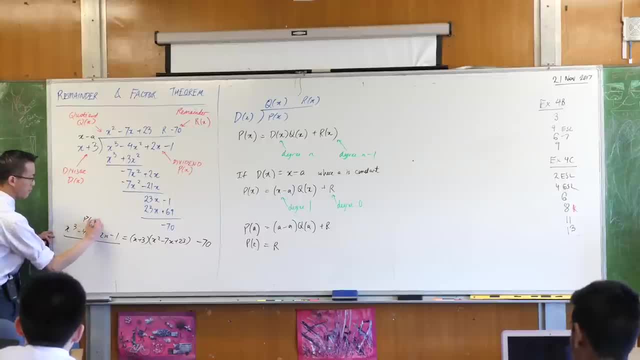 So if this is p of x, then if I put in p of negative 3, let's just quickly crunch this number- What's that going to be? Negative 3, all cubed is going to be negative 27 minus 4 lots. 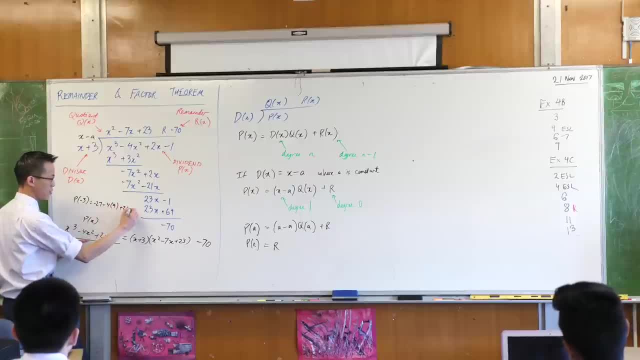 of 9 plus 2. lots of negative: 3 minus 1.. Minus 27,. minus 36,. minus 6,, minus 1.. Looks like minus 70 to me, yes, Which is rather quicker than going through all of this, if